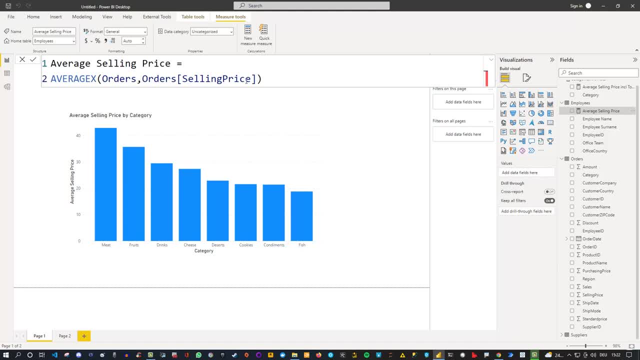 wondering. It's just an average x over the orders table and then I'm showing the selling price for the orders And you might also want to maybe group this first using summarize, for instance, for each order ID, Anything like that. But for now that's not the main point of this video, So how can we? 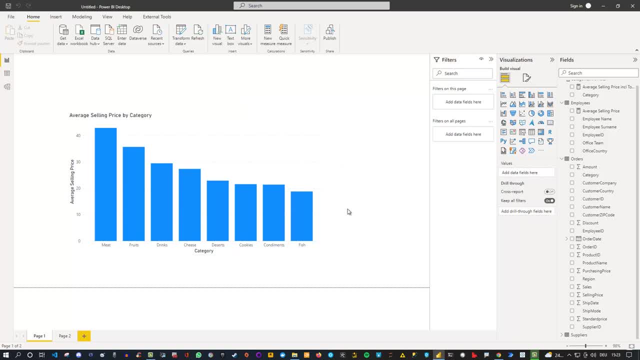 now add the total here. Well, the trick, simply, is that we need to create a table which contains a unique list of our- in this case for me- the categories, as well as one additional entry which is total. So that's what we need. So we need this table. How can we create this table? Well, there are various options. Of course, we could. 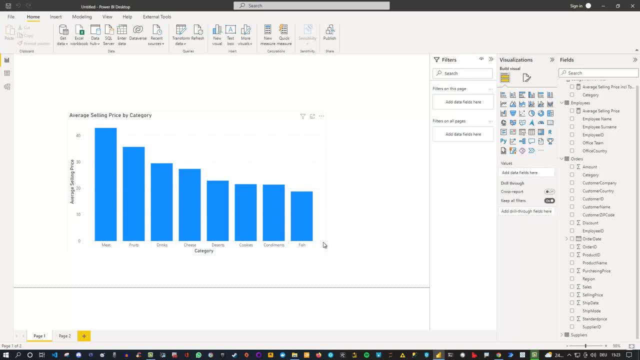 do it, for instance, in Excel or any other kind of tool, and then simply import this table. That could be an option, But we could also do it directly in Power BI using DAX, Because, remember, if you go to modeling here, you have the option not only to create measures but also to create a table. So 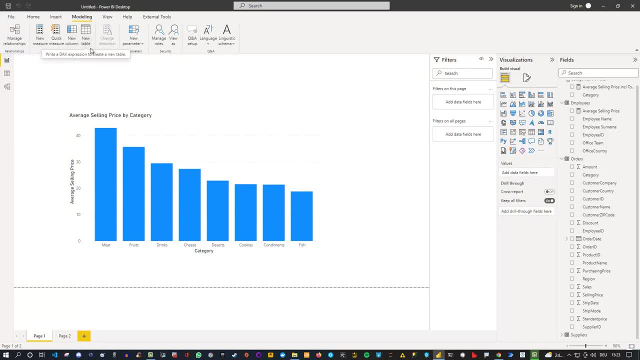 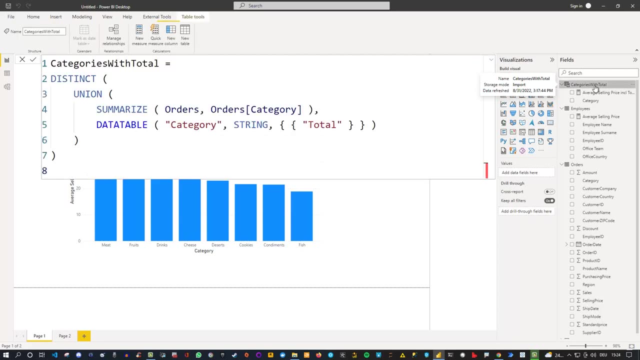 that's what I'm going to do here, And let me show you how that works. This one here, as you can see, with the little calculator icon, is a DAX table which was created by me. It's called categories with total And that's the formula, what it looks like. So what I basically do here is I'm going to 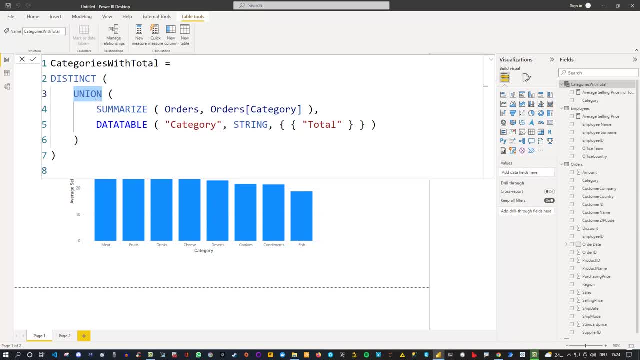 use a union, And the union function allows us to combine two tables, So simply concatenate them and then we can create a table. So that's what I'm going to do here, And let me show you how to do that. So the first table here is: I'm using the summarize function, But you could also. 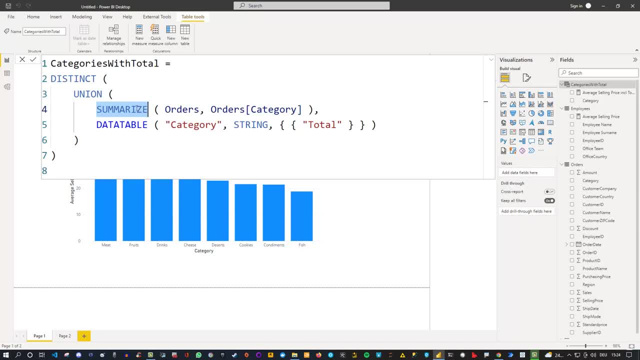 try out different functions, like values, for instance, or anything like that, But what I do here is I use summarize and summarize my orders by the category, which should give me simply a list of categories, And then I also use here an additional function, which is the data table. The data table. 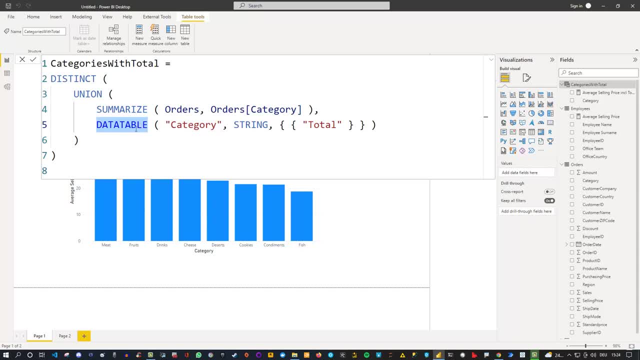 itself is kind of interesting because it allows you to create a table. And then if we look at create a new table and what you do is you specify at first in here- as you can see here- the name- so in this case it's called category- then what kind of data type this table has. in this case it is a. 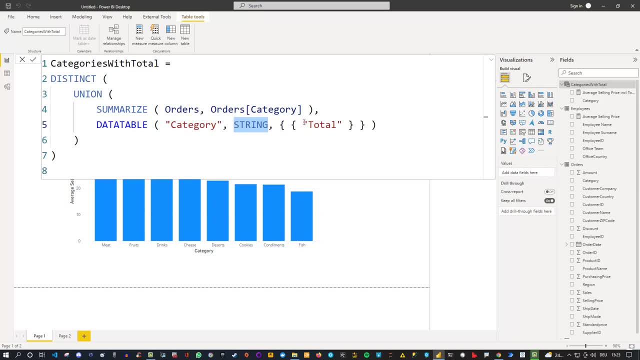 string, because it's text value, and then the specific value itself, which is, in my case, total, and you need to make sure that you have the curly braces here and that's how that works. so what it basically does is with the union. here we first have a unique list of categories from the orders. 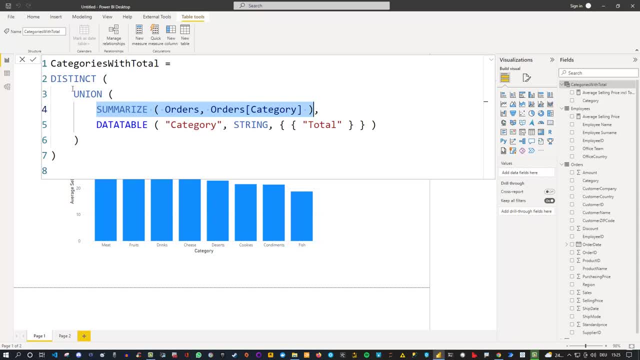 table which is called categories. that is why, for the union, the second table i also called category, and i simply add one specific entry in this table which is of data type string, and the value itself is total, and then we simply- i also wrapped it in distinct, but maybe that's not necessary especially- 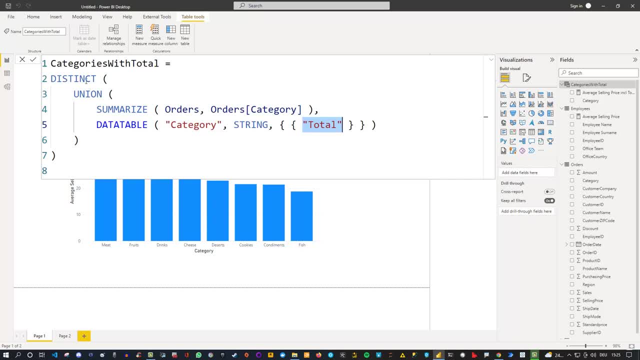 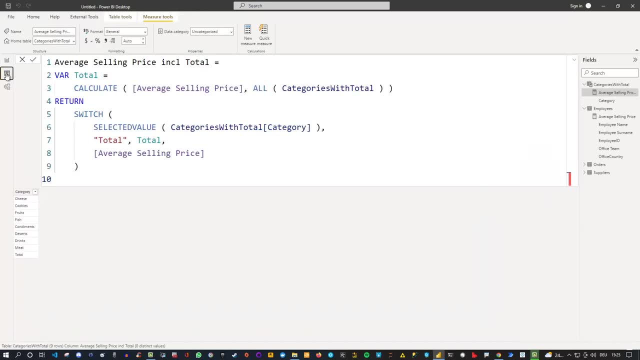 if you do not have any duplicates. but nonetheless, i did that and let me show you the result of this. so if i close this now and go to the data view in here, this is where you can actually see what the result looks like. so it's a unique table which is called 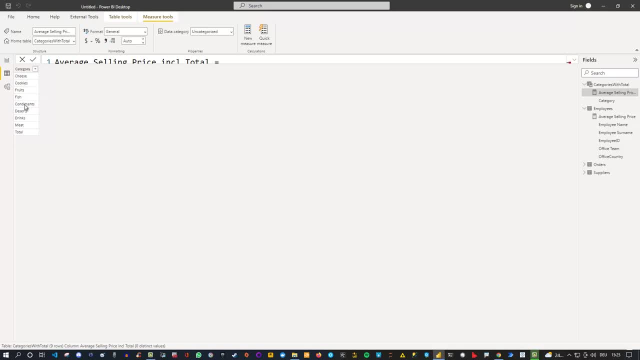 category and it has a unique list of the categories, and especially take a look at this one here. unfortunately, right now i can't zoom in, but if you do it yourself, you'll see that there's a one additional entry, which is total, and that's exactly what we get by creating this function. 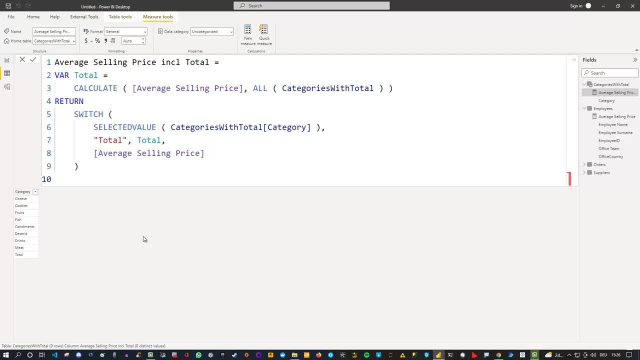 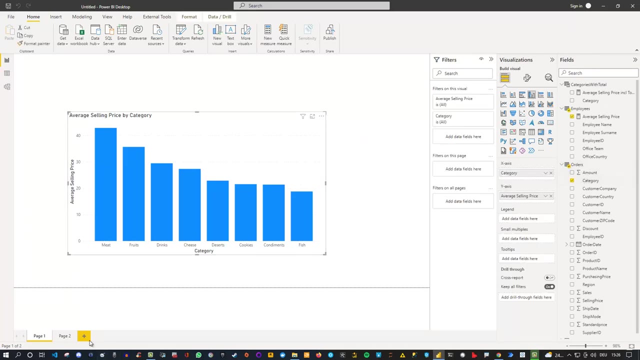 here. so this text calculation which returns a table. so that's the first thing we need. so now we have our category table including the total. so that means that instead of using the default category from my orders table here, i can now add in here another visualization type which is in this case coming: 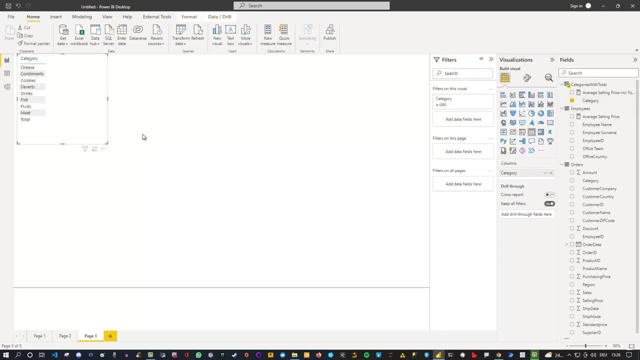 from the categories with total, so i can select this category now and also choose a bar chart like that. okay, here we go, and of course we also need some kind of entries here. right, and what we can't use, of course is right now the average selling price, because if i would use this one here, 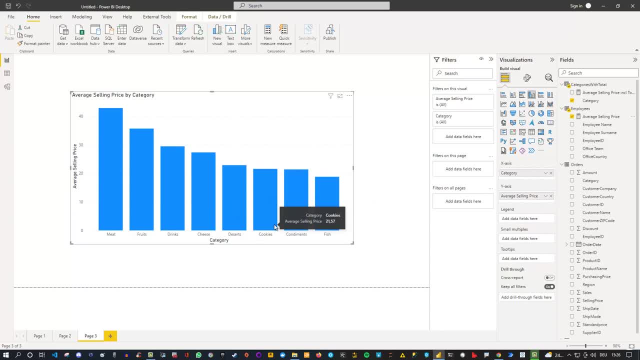 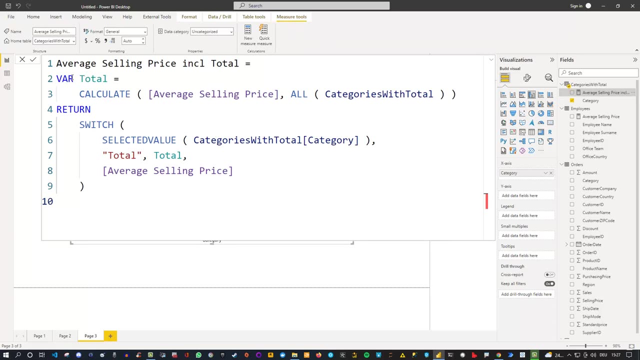 i'd see there is no total right, because the total here is not included for, or the selling price is not there for, the total. so what we need instead is we need to modify this measure a little bit, and that's what i did here, and let me show you the result. so i'm using variables here, because what i 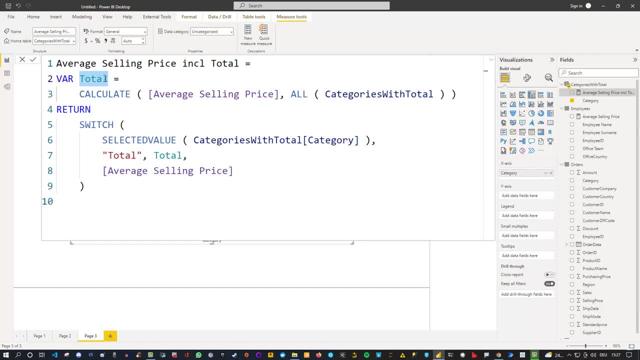 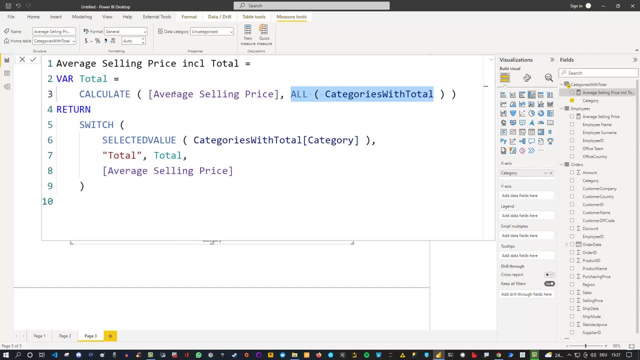 have on the x-axis. so i'm sure that i include all the categories. that's what i'm using to calculate here, because i need to modify the filter context, and that's what i do with the all function here, and then i simply use a switch statement and take a look at the selected value of the category state. 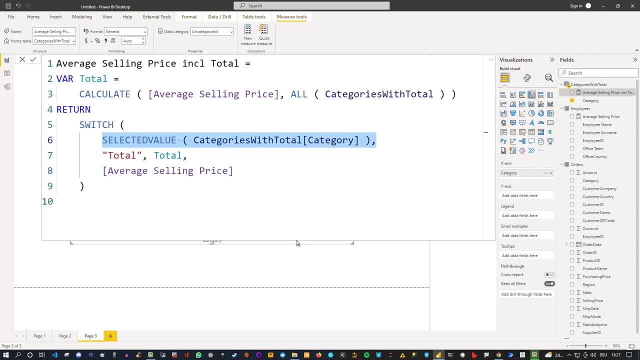 total, which is simply each value in our x-axis, and if the value is total, then I like to show the value across all categories. so this up there. otherwise I'm using my default measure, which is the average selling price. that's all what we do here, so you don't have to use the variable if you. 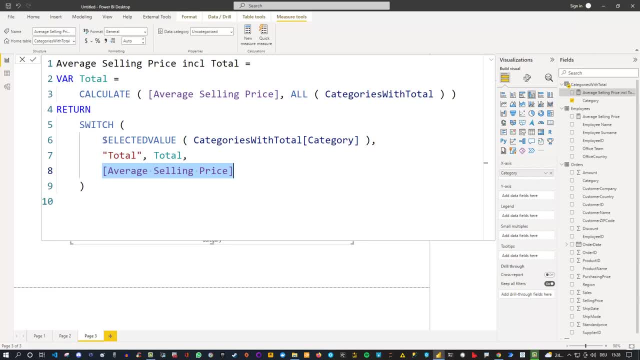 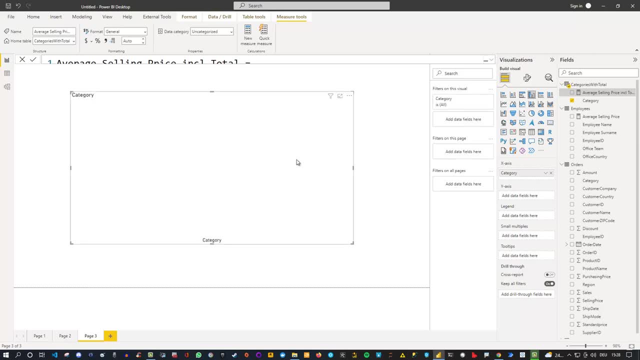 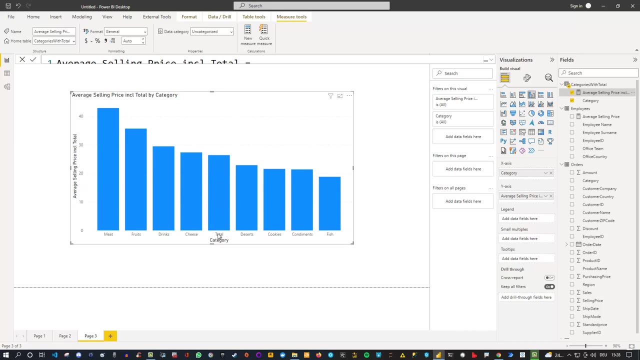 don't like to, but I think it's quite cleaner writing DAX this way. so that's why I chose to do it this way. and after this- let me just close this here- make small again, and if we put this in the visualization, let's do that, let's put this inside. now we see we got one new bar, which is here: 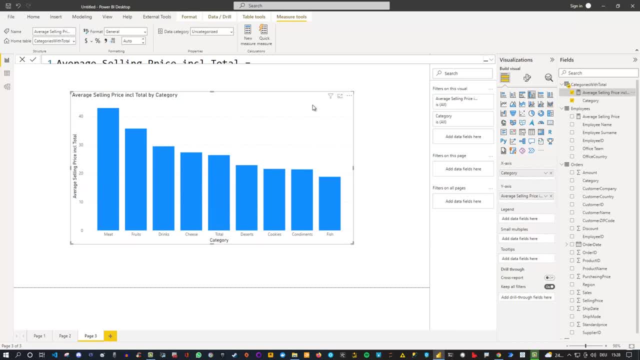 which is the total bar. hope you can see it. maybe it's a little too small, but if I let me just check that here, if I go to the x-axis here and I would make the bolts or maybe a little bit bigger as well, you should hopefully see that there's a total in here, right? so that may be a little too big, or. 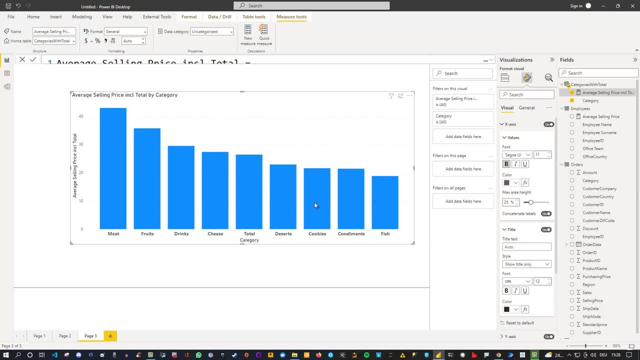 make it bigger, like this, and if I go to the x-axis here and I go to the x-axis here and I go to the like that. so, and the only thing which might disturb a little bit is that the total is currently in the middle. I get that, but let's take a look at the sorting options here and 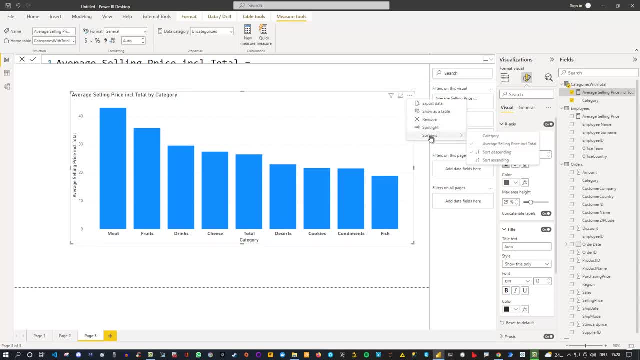 actually by default, because the total is at the end. we should be able to sort it here not by average selling price, but let's choose the category. here and now we can see that the total is at the beginning and this is because by default it's sort of descending here. but if 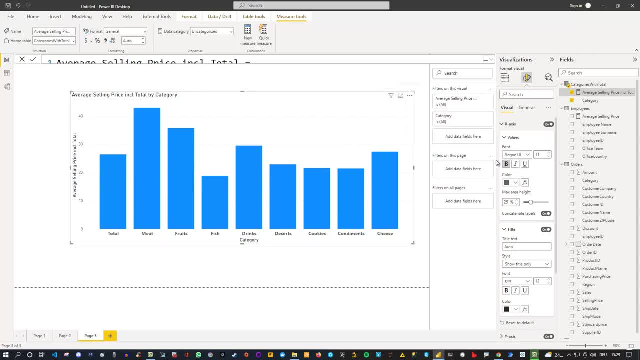 I go to sort access now and click on sort, ascending like that. then we see that now the total is at the beginning and this is the last value in here, the bar, and of course, you can now play around with the color. if you want to do that, let me also maybe go here and also add the labels.